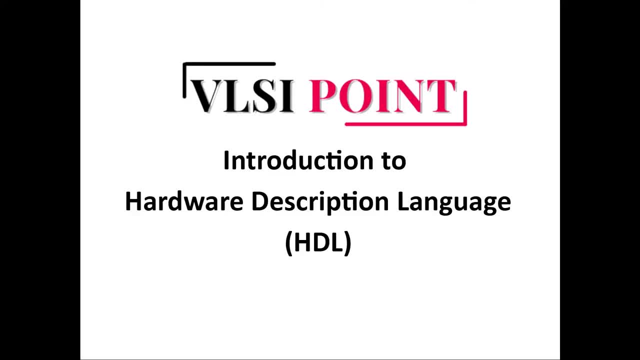 Hello everyone, this is Shweta and welcome to VLSI Point. So, guys, this is the first video of complete Verilog course in English. So in this course I am going to cover all the Verilog topics, from basic level to advanced level, in very simple words. So if you are a beginner and you are just 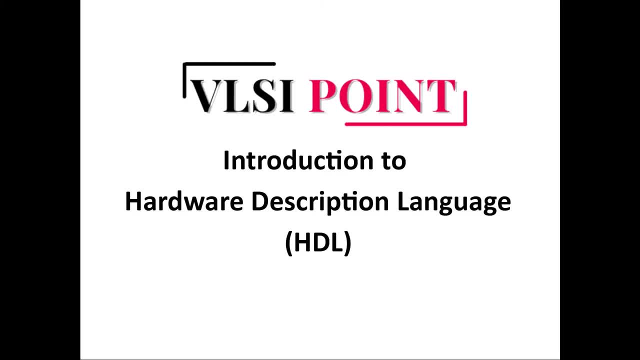 planning to learn Verilog. you just want to build your concept, then you must join this course. Even if you have some basic idea about Verilog, but still you are not confident with some advanced topics, then you should also join this course. So in this lecture we will learn about HDLs. 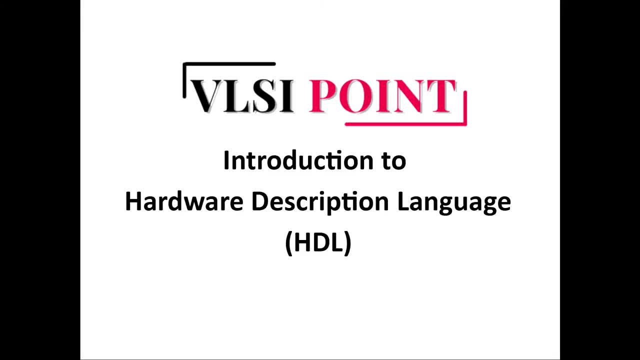 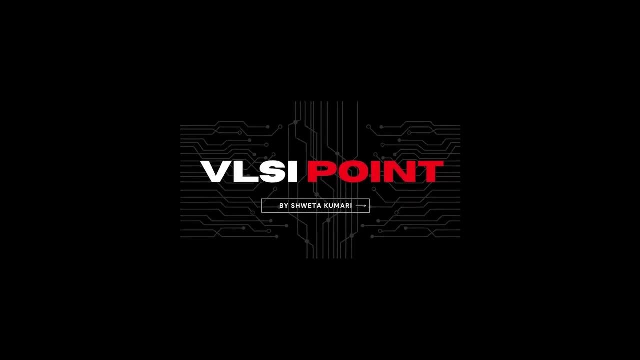 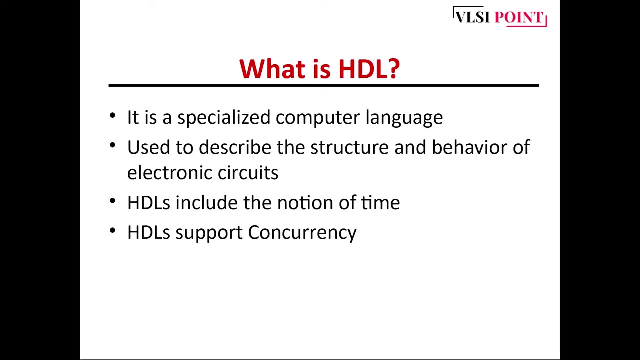 What is HDL? What are the advantages and why we should use HDL? We will learn everything in this lecture, So without any delay, let's get started. So HDL stands for Hardware Descriptive Language. It is a specialized computer language. 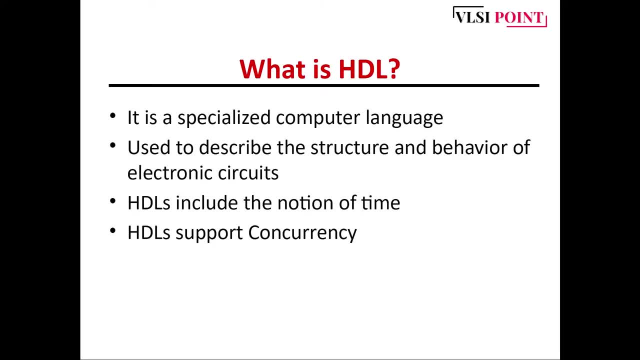 which is used to describe the structure and behavior of electronic circuit. Whenever we are talking about HDLs, directly or indirectly, we are talking about a piece of hardware, So this language is related with hardware circuits In early 70s, when we didn't have HDLs at that time, pen paper and 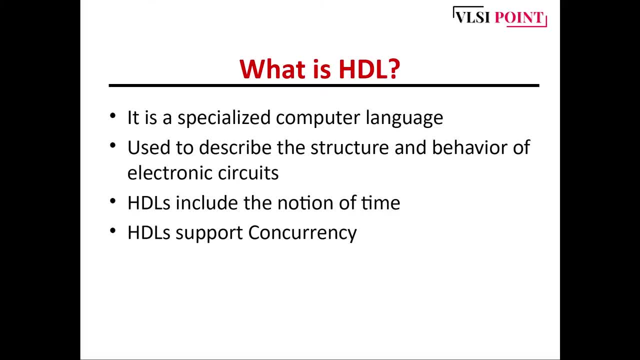 drafting tables were used to describe the specification of the circuit. Since now we have HDLs, so we can simply translate our code into HDLs, So we can simply translate our code into the digital circuit. HDLs include the notion of time and it also supports concurrency. 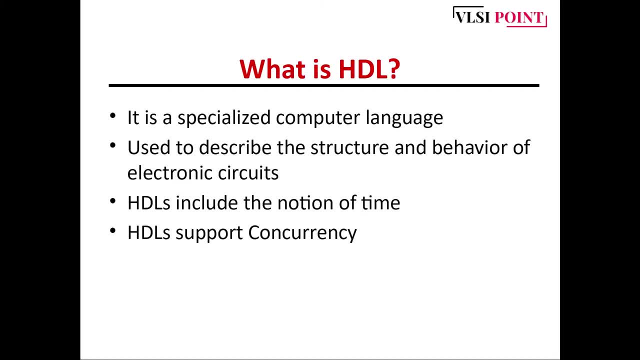 So this is the property of HDL. Whenever we are talking about notion of time, so it is basically related with the time delays of digital circuit In real time. each and every hardware circuit have some time delay and HDLs include that time delay. So this: 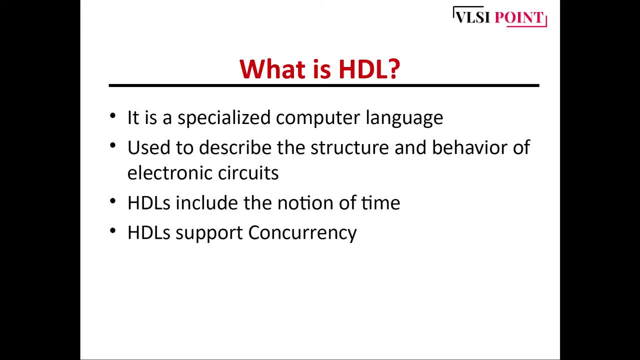 is the property of HDL. talking about another property, which is concurrency. So concurrency is nothing, but whenever two things are happening simultaneously, that is called concurrency. Suppose, in a circuit there are two blocks and both the blocks are executing at the same time. so this is the example of concurrency and HDLs also support the concurrency. So 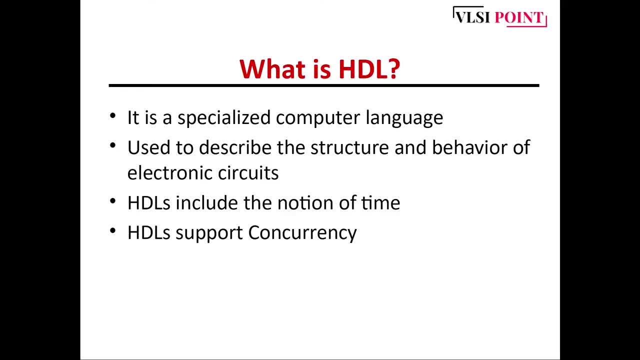 it is a concurrent language. However, if we are talking about other programming languages like C and C++, so these are not concurrent languages. these are sequential in nature. So this is all about HDLs, Verilog and VHDL. both are hardware descriptive language, so 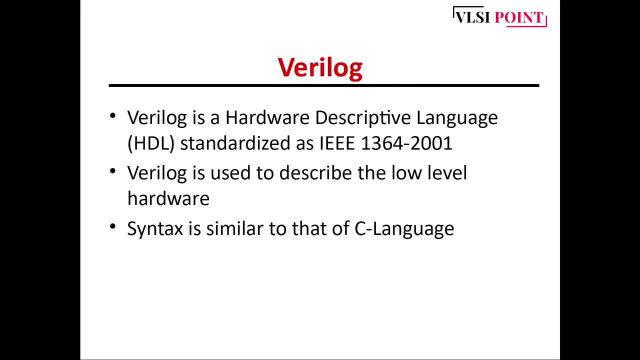 we will start with Verilog. So Verilog is a hardware description language and the current state of the hardware description language is the hardware description language. So the standard is IEEE 2001.. Verilog is basically used to describe the low level hardware. Actually, 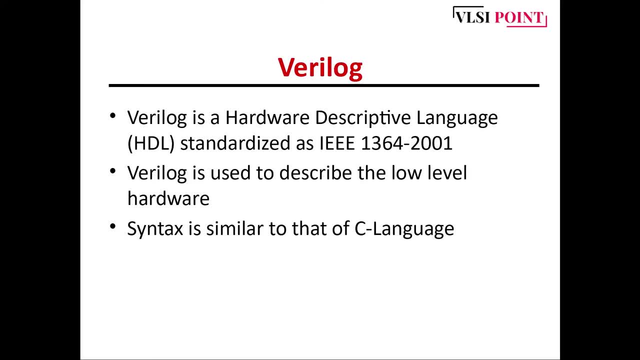 Verilog is a very flexible language. In Verilog there are some predefined basic gates and digital circuits which are already saved in digital library of the Verilog So we can directly use those blocks and that are known as primitives. Verilog is a very much similar to C language whenever we are talking about syntax, But 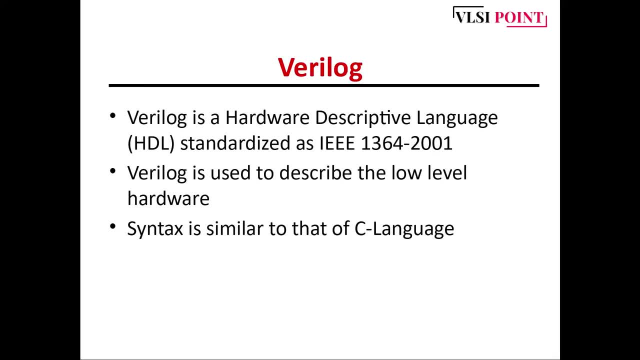 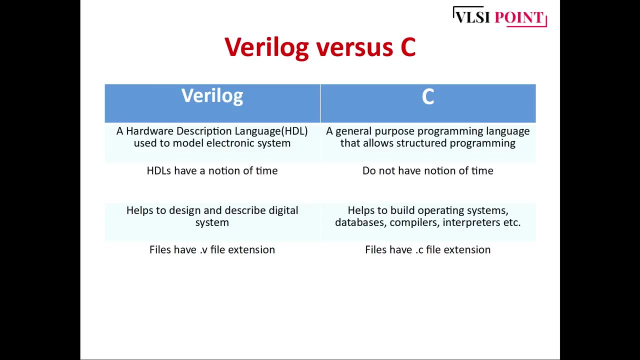 still, there are some difference between Verilog and C language. So let's see what are the difference. Verilog is a hardware description language which is used to model electronic system. However, C is a general purpose programming language which allows the structured programming. HDLs have notion of time, However C language don't have the notion of time. Verilog helps. 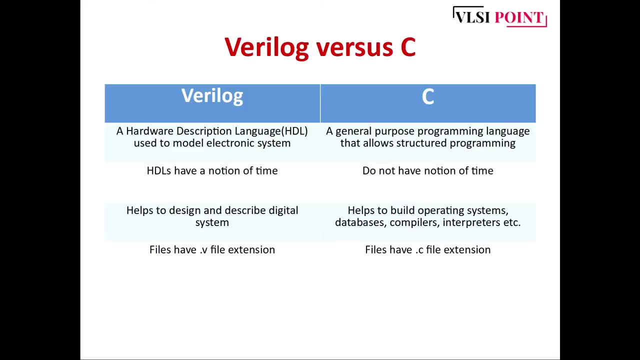 to design and describe the digital system. However, C helps to build operating system and database compilers: interpreters. In case of Verilog, the file extension is v. In case of C language, the file extension is c, So these are C language. 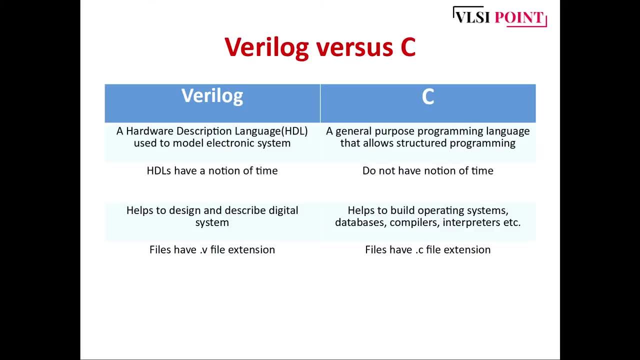 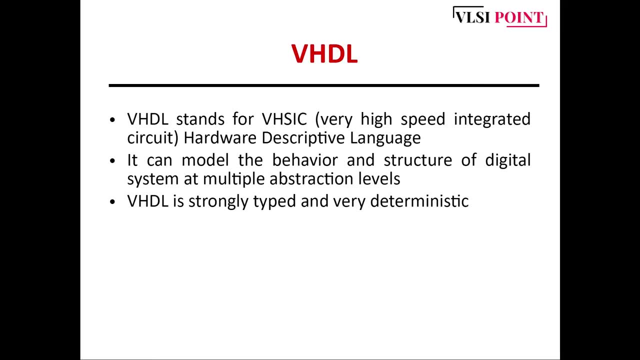 Now we are moving towards VHDL. So VHDL stands for VHSIC. That means very high speed integrated circuit hardware description language. VHDL are basically used to model behaviour and structure of digital system at multiple abstraction levels. VHDL is a kind of strongly typed language and it is very deterministic. VHDL is an old 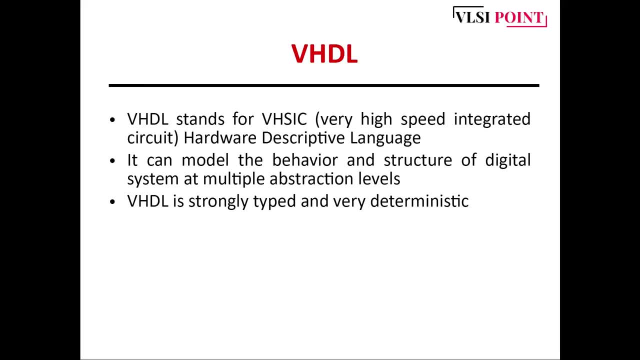 language and it has developed in 1980s. VHDL syntax is non C type and the advantage of VHDL is that we can easily fix the bugs in VHDL as compared to Verilog. So these are the advantages. But, yes, VHDL is strongly typed, mean to say whenever we are writing the code in VHDL. 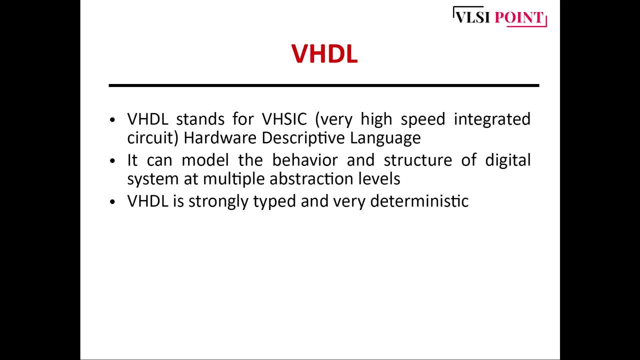 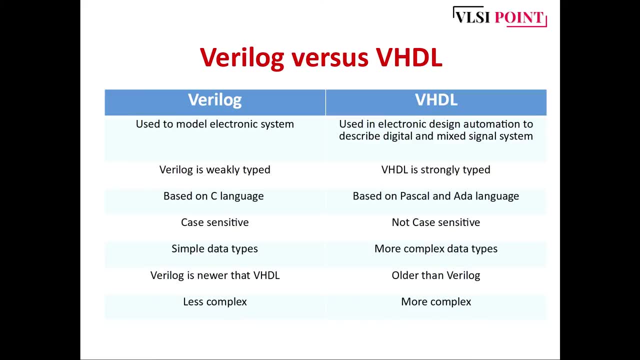 So code will be a little bit long as compared to Verilog. So now we are going to see some differences between the Verilog and VHDL. So Verilog used to model electronic system. However, VHDL used in electronic design automation to describe digital and mixed signal system. 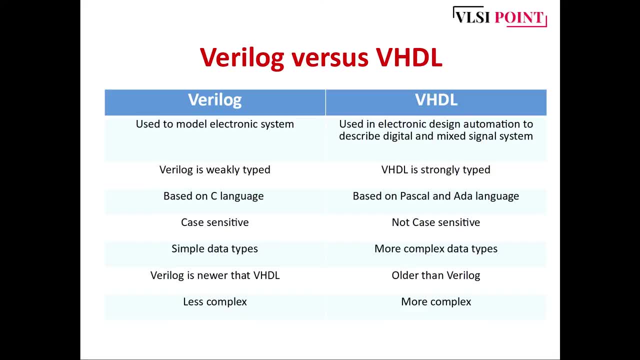 Verilog is weakly typed. However, VHDL is strongly typed. Mean to say, VHDL is more strict about the syntax. Verilog is based on C language. Syntax is very much similar. However, VHDL is based on Pascal and ADL language. Verilog is case-sensitive, VHDL is not case. 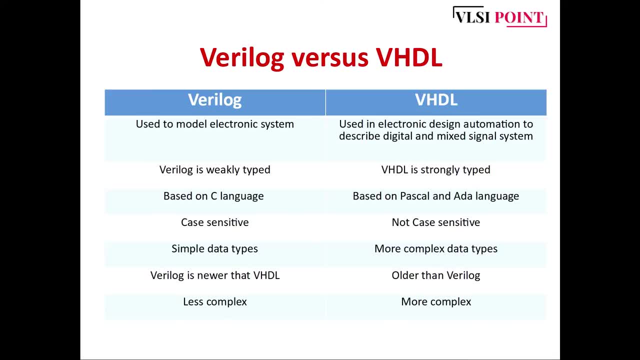 sensitive In Verilog. we have simple data types. In VHDL, data types are more complex. It's not called VHDL and its like this in the last one, So it's case sensitive. VHDL is not case sensitive In Verilog. we have simple data types in VHDL. 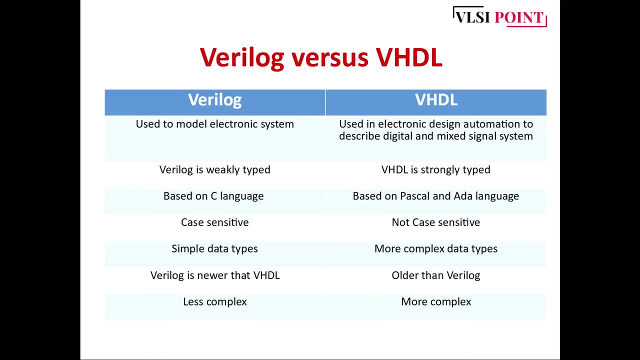 Data types are various. In the case sensitive, VHDL is case sensitive and it's not case sensitive complex. Verilog is a new language. Standard is 2001,. IEEE 2001.. However, VHDL is an old language and it has developed in 1980s. Verilog is less complex in nature. VHDL is more complex in nature.